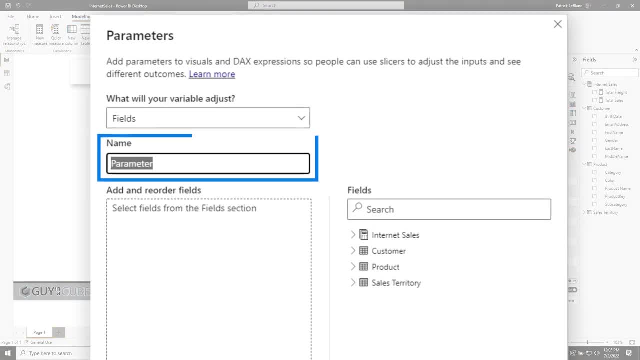 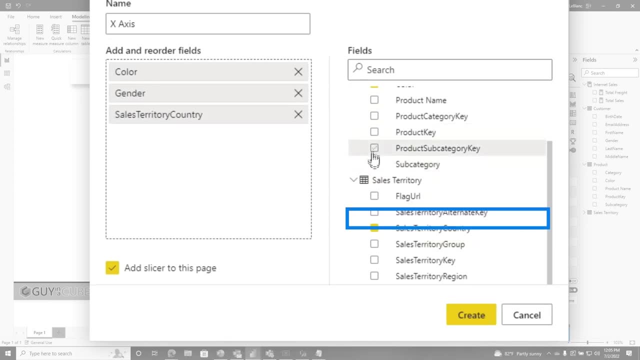 choose new parameter. We're going to choose fields And we're going to call this one X axis. We're going to choose color, We're going to choose gender, We're going to choose country and even subcategory. I'm going to click create If you're not familiar with the field parameters. 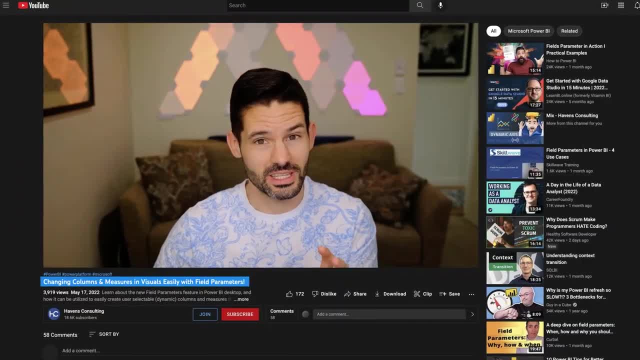 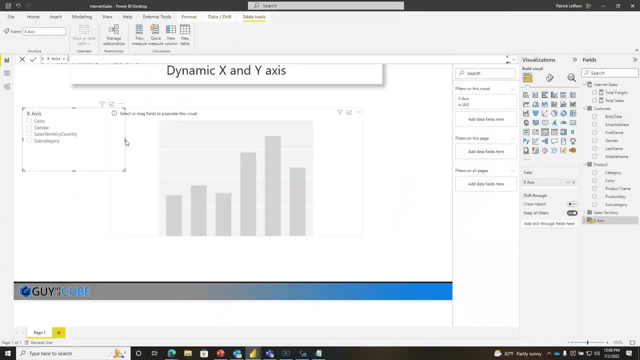 there's tons of videos, tons of content out there and you should go read the documentation. It's a great new feature that was released recently as of the recording of this video in Power BI. When you create that field parameter, it automatically adds a slicer to the page And 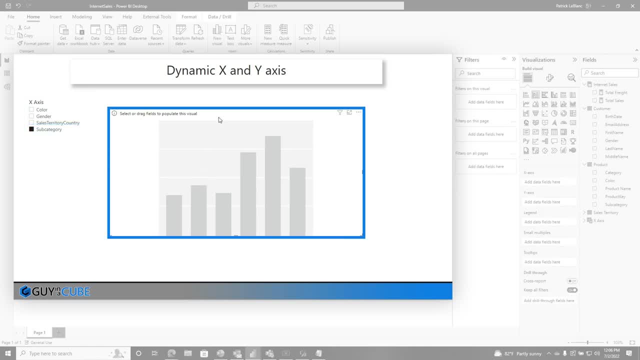 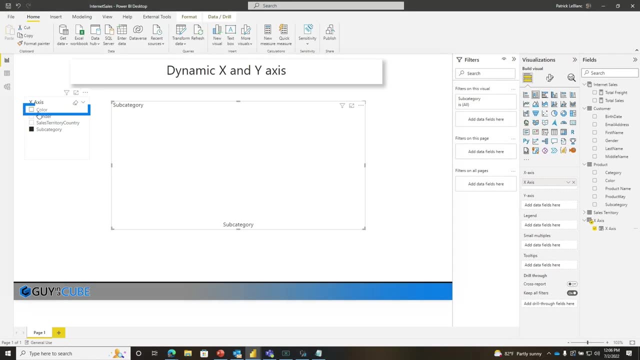 what I'm going to do is I'm going to choose subcategory, go back over to my column chart here. I'm going to take that particular column from my field parameter and drag it to my X axis, And so you can see if I choose it. 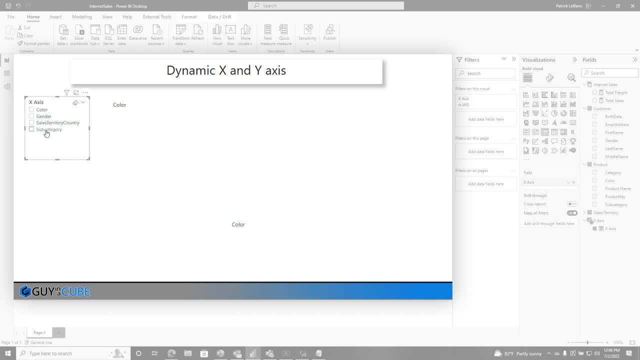 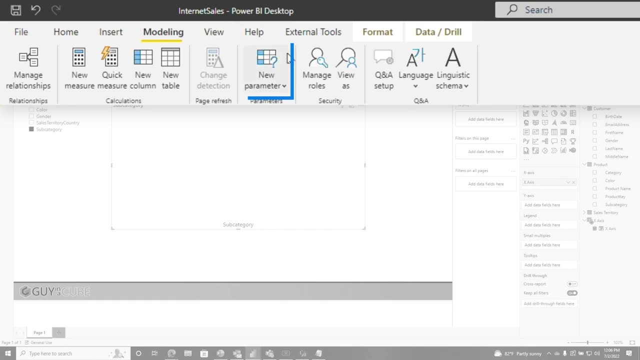 right, it's changing the name of it, the label for the X axis to different selections. And then what would you do for the Y axis? Well, create another field parameter. So we're going to go back to modeling and we're going to choose new, new parameter fields. We're going to call this: 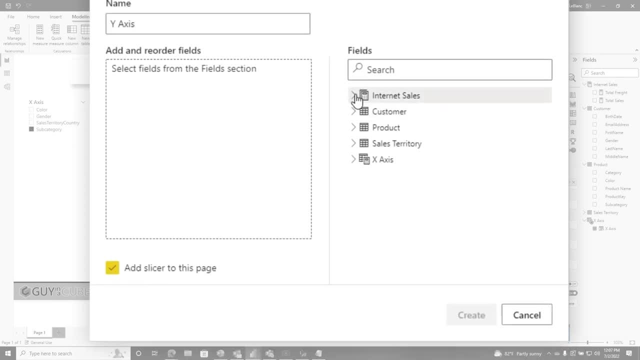 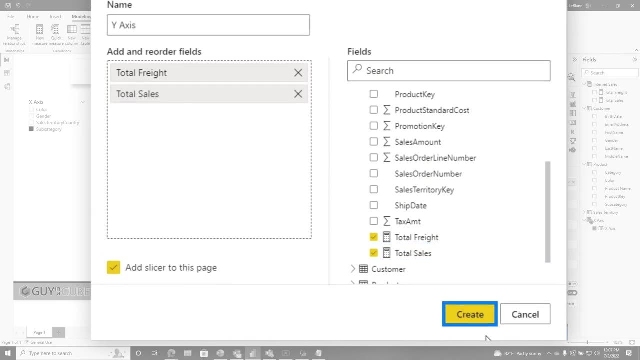 one, the Y axis- And then we're going to add our measures here, because typically on the Y axis you have measures. So we're going to add total freight and we're going to add total sales. If you keep this checkbox checks, it'll add the slicer to the page. So I'm going to go ahead and 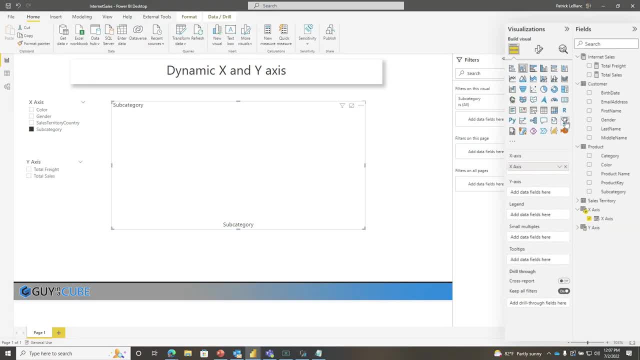 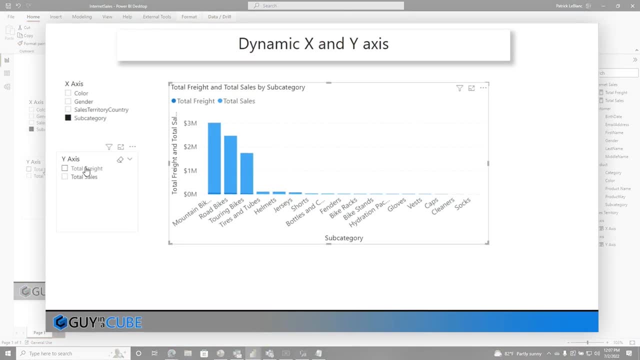 and there's my Y axis slicer. So I'm going to go back to my stack column chart and I'm going to add this guy right here to the Y axis. And now you can see both right: Total freight and total sales. If I choose total freight, my Y axis is now based on total freight. If I choose total sales. 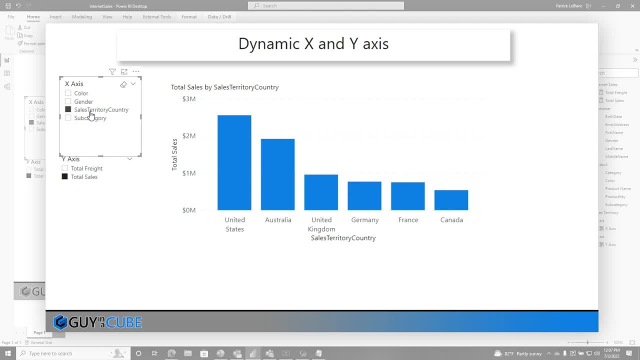 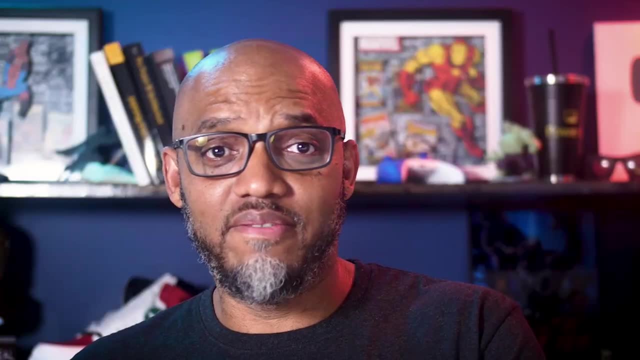 it's going to be based on total sales And if I choose color, gender, sales territory, country, subcategory, it just all works and it's completely dynamic. All right, what do you guys think Now? you have dynamic X and Y axis on different visuals and 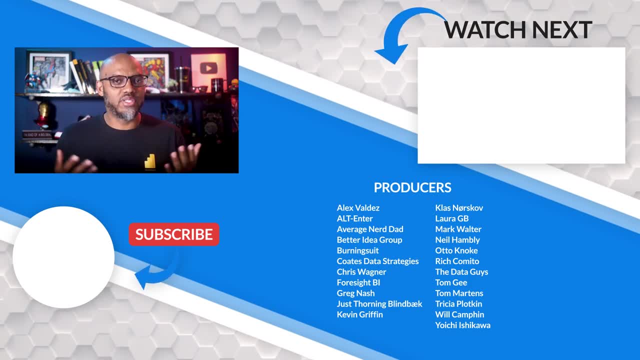 Y, Have you tried this before? Is this something you've been thinking about and you just couldn't solve? I'd love to know. Let's continue the conversation Where, In the comments below. If it's your first time visiting the Guy in a Cube channel, hit that subscribe button If you like my. 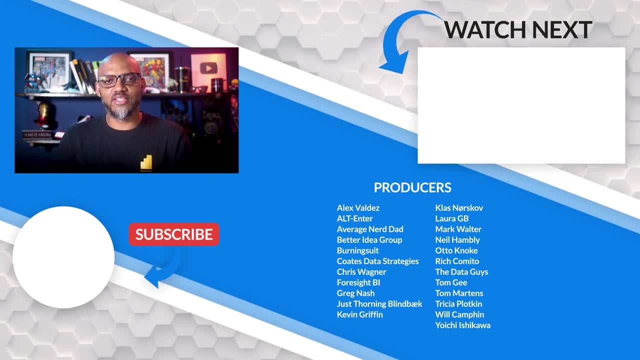 video. give me a big thumbs up, As always, from Adam and myself. thanks for watching. See you in the next video.